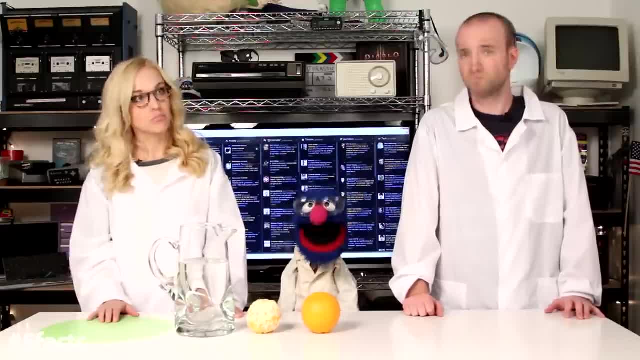 say the heavier one, which would be the one with the peel. Let's start with the peeled orange. Ready? Yes, Good thing I'm wearing these goggles. Hahaha, Would you look at that? No, Just look. You can't see it. It's a blue orange. I'll just cut it. You can't see it. I'll just cut it. I'll just cut it, Okay. 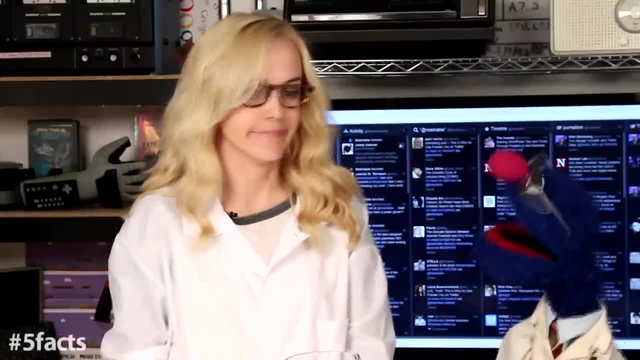 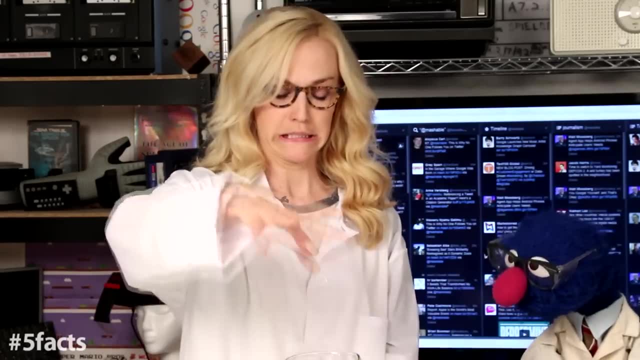 Oh, good thing I'm wearing these goggles. Ha ha, ha ha. Would you look at that? It is sinking. Now let's test the unpeel. OK, Come on, Molly, It is floating. It is floating. Look at that, Danny. 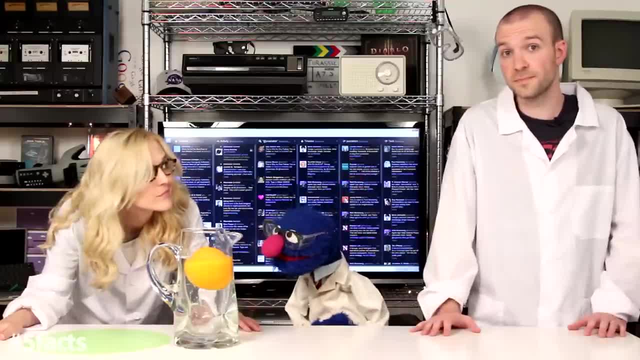 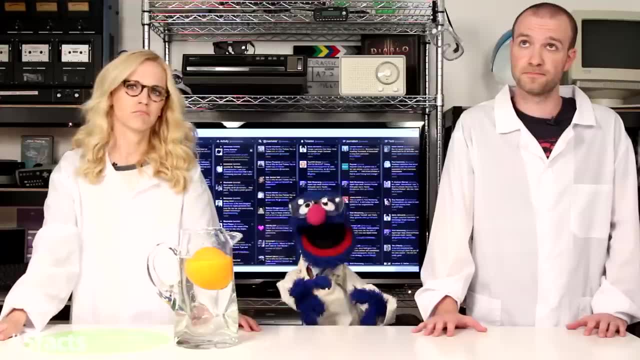 It is floating. How long do we have to wait until it sinks? Well, it'll never sink, Never. But why? There's air in the peel that makes the orange buoyant. So the peel is sort of like the orange's life jacket, huh. 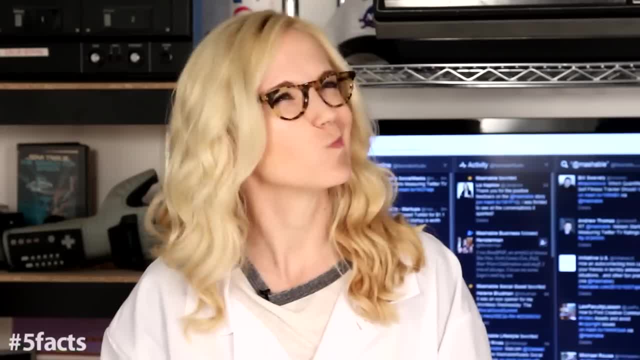 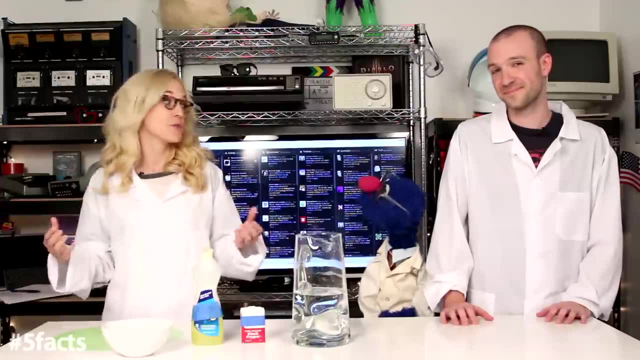 Exactly. Next time I go swimming, all I have to do is wear an orange peel. I don't think that's no. Here's a really neat science experiment to impress your friends back at Sesame Street. Oh, I'd love to impress my friends back on Sesame Street. 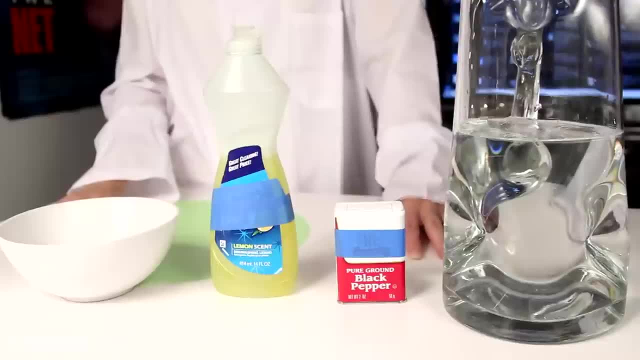 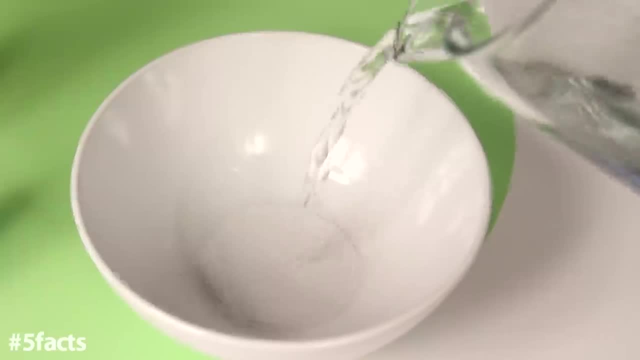 with neat tricks. Ha ha ha ha. All you need is a pitcher of water, some pepper, some dish soap and a dish to put it in. We're going to make the pepper scatter really fast. Let's start with pouring the water into the dish. 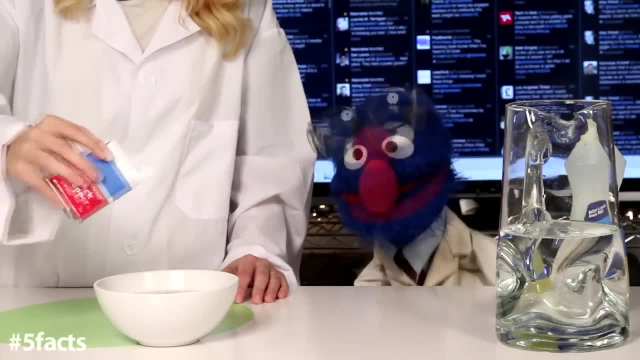 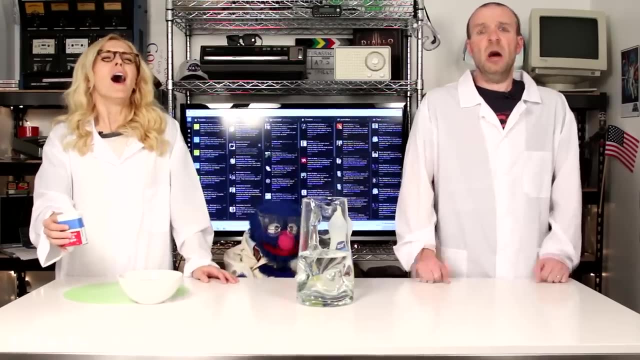 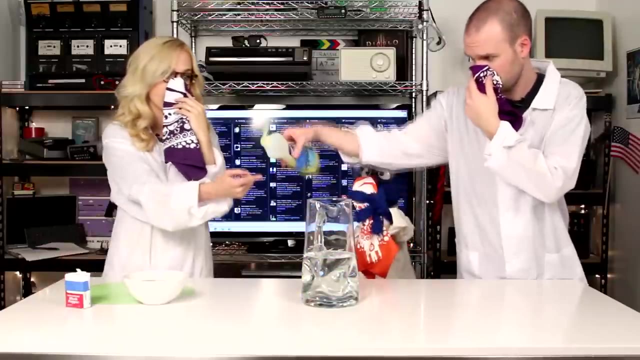 And now we pour the pepper. Ah-choo. Oh, sorry about that. Pepper made me snap Ah-choo, Ah-choo, Ah-choo, Ah-choo. And now you just put dish soap on your finger. 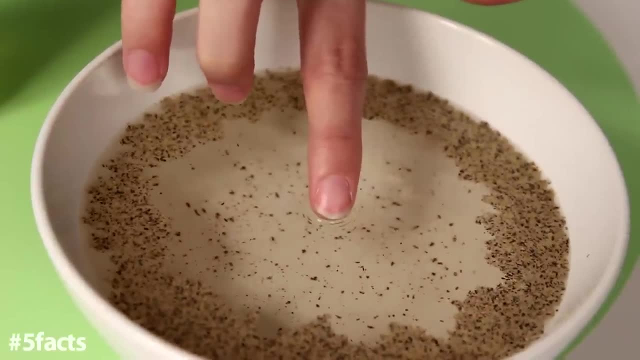 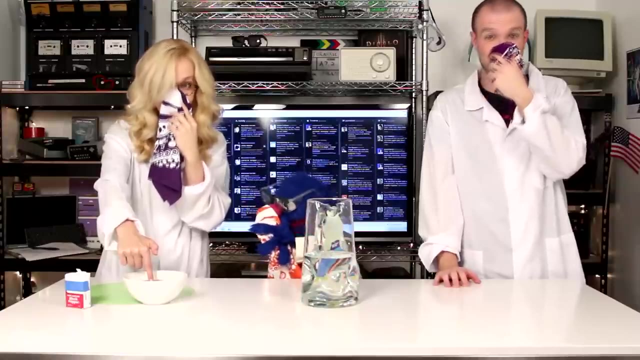 And three, two, one. Wow, I haven't seen anyone run away from soap that fast since Big Bird tried to give Oscar the grouch a bath. Ha ha ha. How does this trick work? It's all about surface tension. surface tension is the force that allows water to bulge on the top. 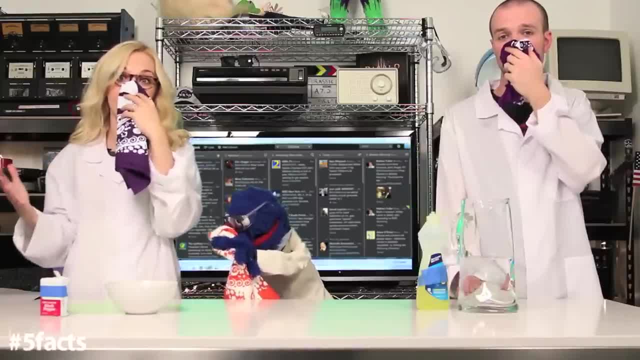 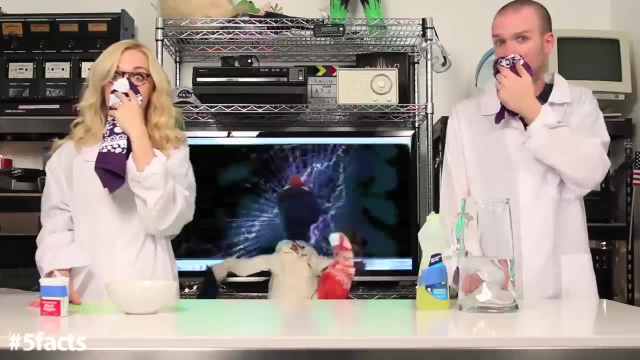 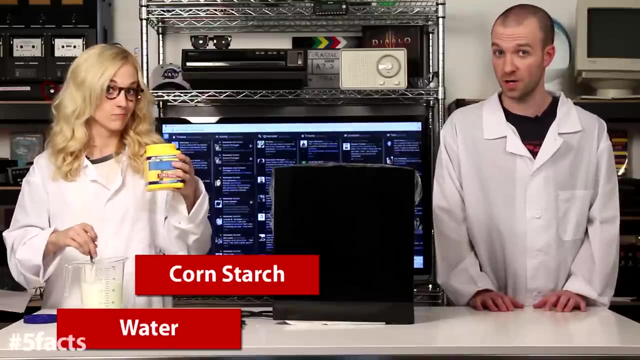 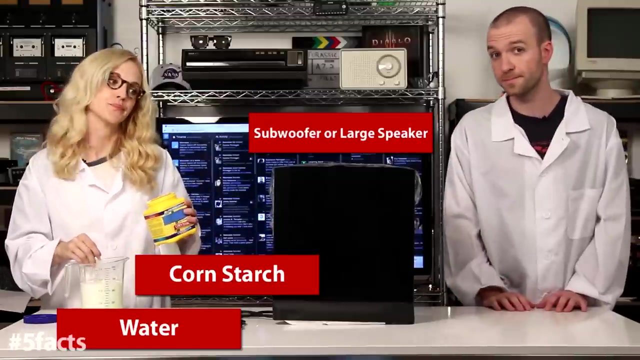 the dish. soap lowers the surface tension, which causes the water to spread out. the pepper then moves to the edges. that is amazing. for this experiment, we need to mix cornstarch and water. guys, are you sure this needs to be here? yeah, this is a subwoofer. we need it for the experiment. this stuff is called oo black. 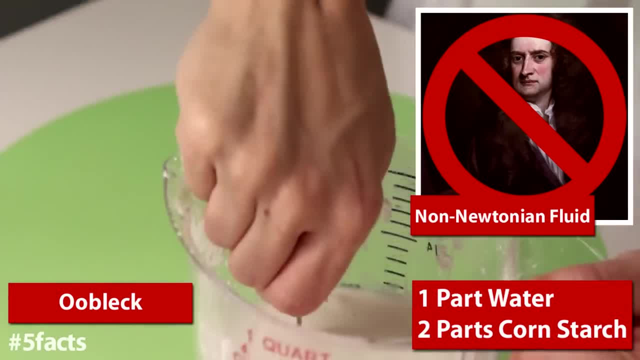 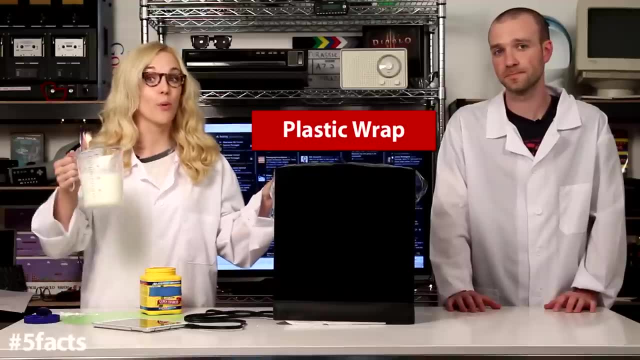 it's a non-newtonian fluid that has properties of liquids and solids. if you touch it it feels like a liquid, but if you pinch it it feels solid. cover your subwoofer with plastic wrap and then you're gonna pour in your cornstarch and 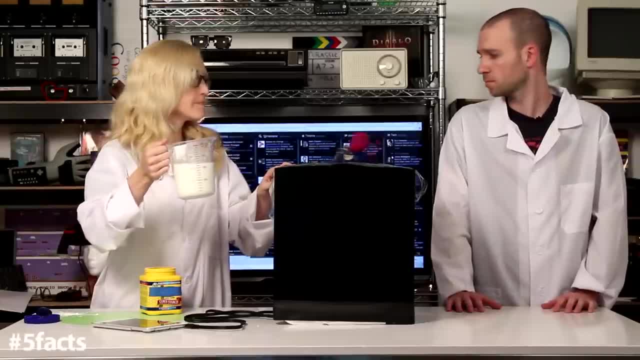 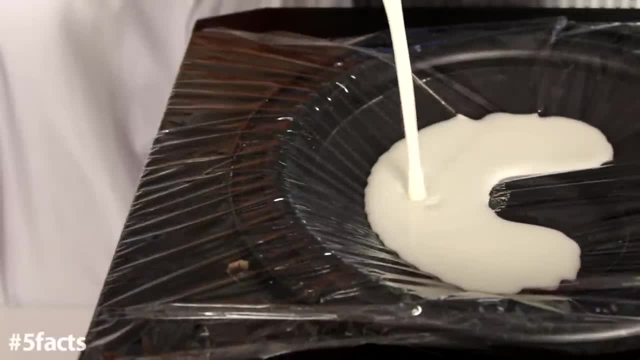 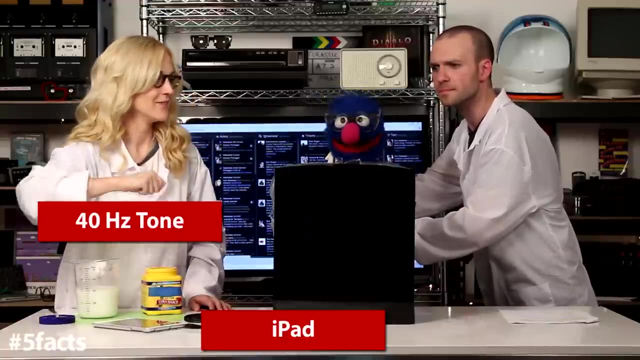 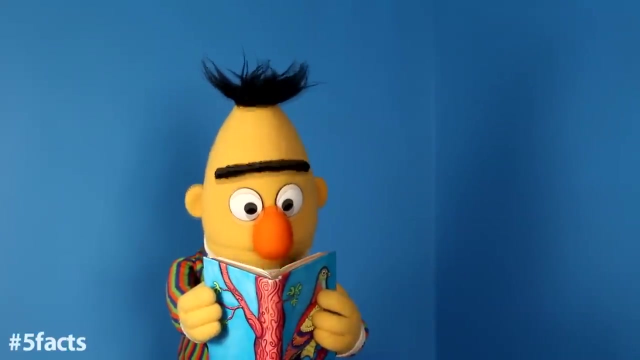 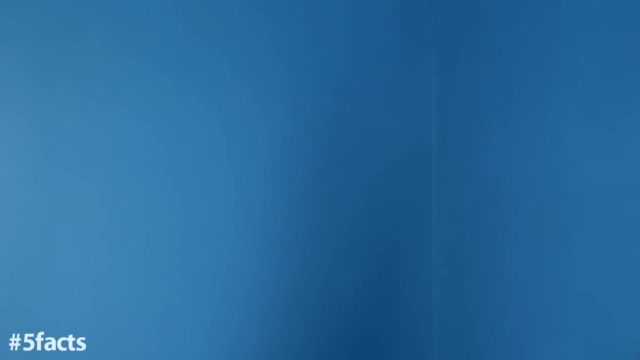 water mixture. I want to see. I want to see Matt. oh yeah, sure, sure, here we go. sound waves have the same effect. the pressure of the sound waves on the oo black gives it solid properties. now we're going to play a 40 Hertz frequency. what is that 40 Hertz? hey, hey, will you kids turn down? 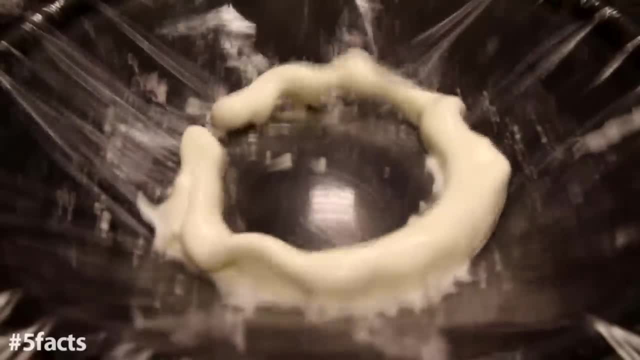 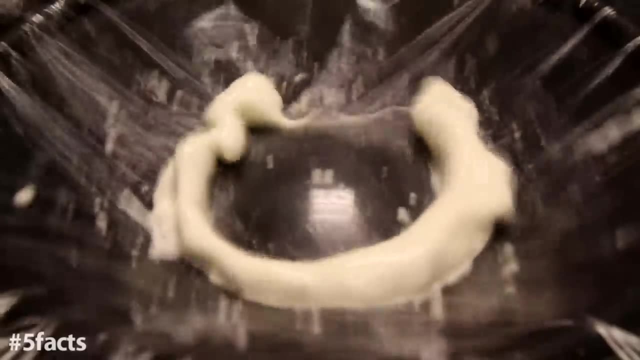 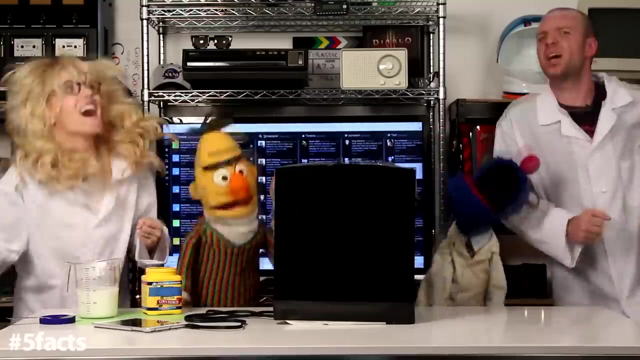 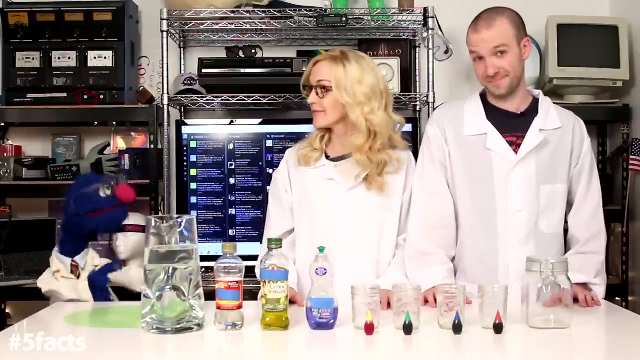 your music. I'm trying to read: is that black? it is, Bert, I think you. black is my favorite non-newtonian fluid. we're having a black dance party. you want to join? yes, hey, Annie, is this dubstep? I think so. did you know you can make a rainbow right in your own kitchen? no, a rainbow, oh I love. 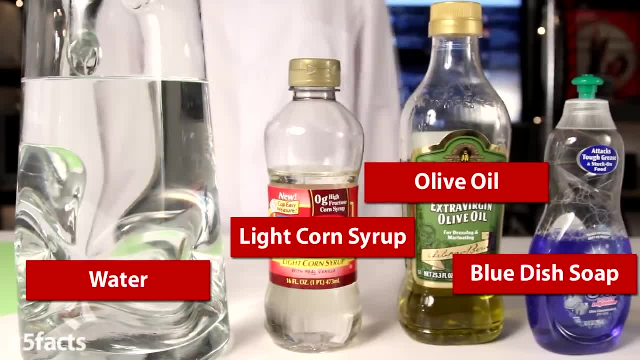 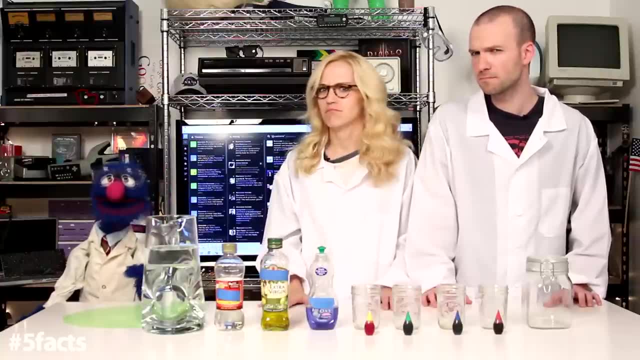 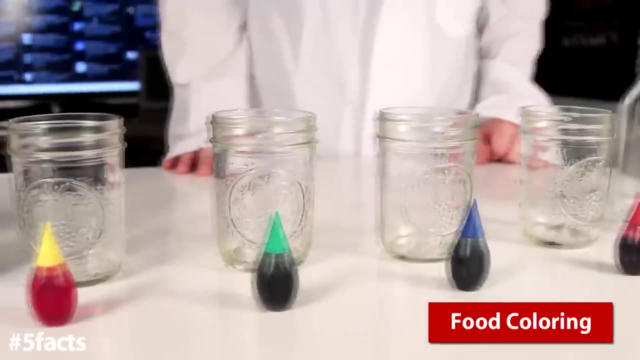 rainbows. they're so cute and adorable. all you need is water, corn syrup, olive oil, blue dish soap. are you sure you're not bringing back the dinosaurs, because this looks an awful lot like my experiment? no, it's definitely a rainbow experiment. let's get started. add food coloring to. 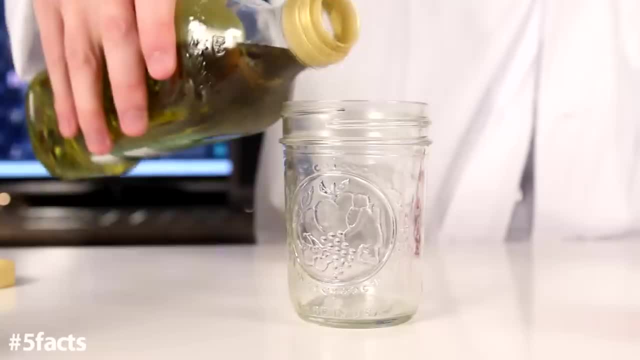 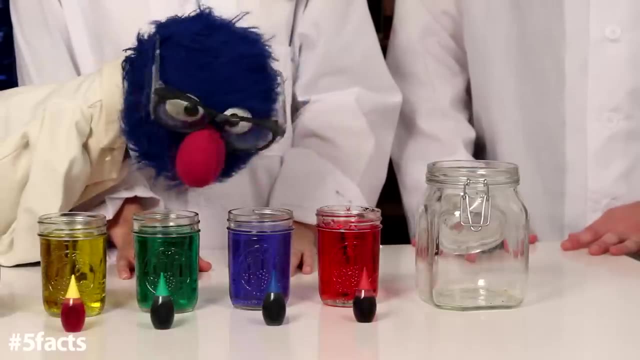 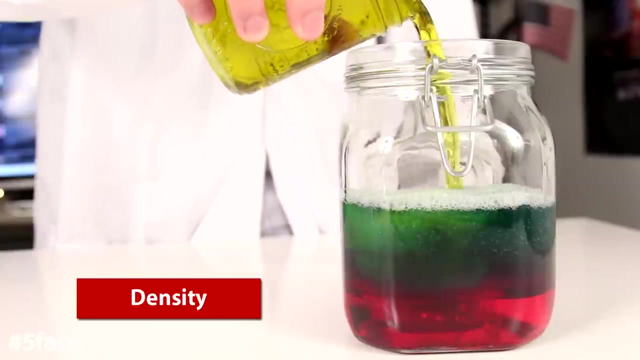 all your materials: red to the corn syrup, green to the water, olive oil is already yellow and the dish soap is already blue. pour your rainbow in this order: red, blue, green and yellow. the reason it works is because each liquid has a different density and certain liquids refuse to mix. thus we get all the layers of the 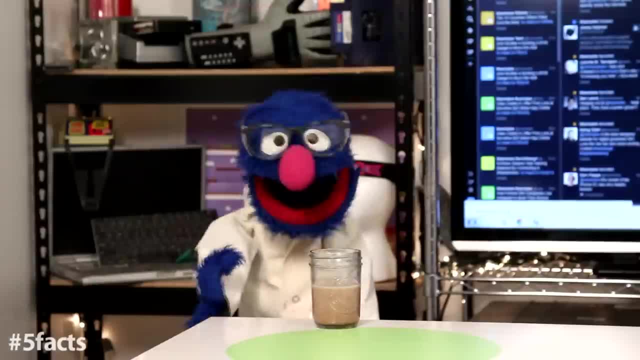 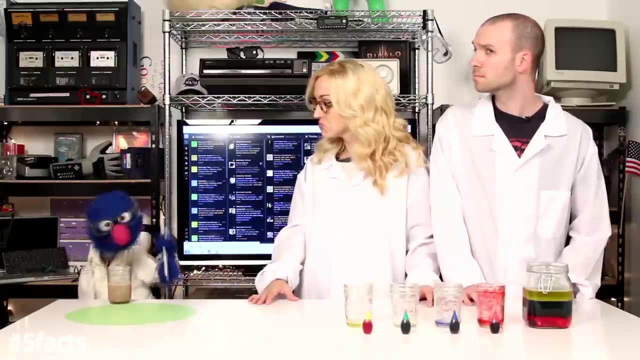 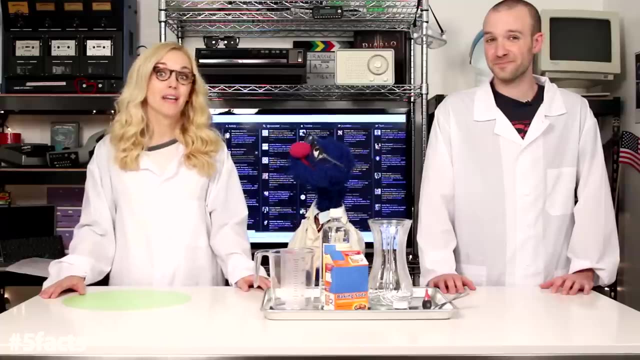 rainbow. there you have it, tada, tada. it's done, Grover, why is yours brown? oh, a good little. you see, I just made myself some chocolate milk. mm-hmm, in this experiment, we're gonna make a sparkly volcano. this is the one with the glitter. is this the? 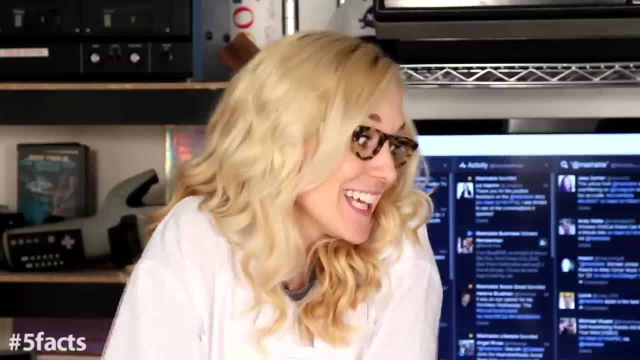 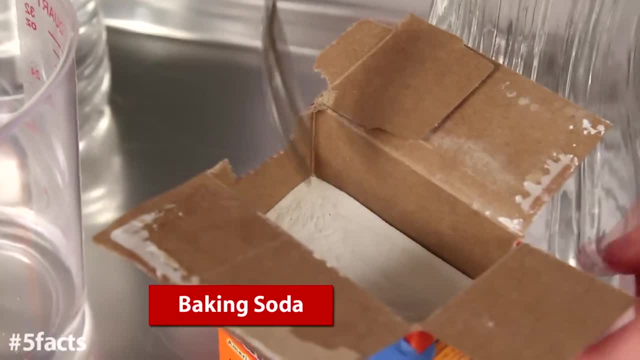 one with the glitter. I've been waiting along for the glitter. is this the good? it the one with the glitter. okay, just look, let's just look. focus on the experiment. okay, you'll need baking soda and a vase pour that baking soda right in there. then you want to add some and to pour��.